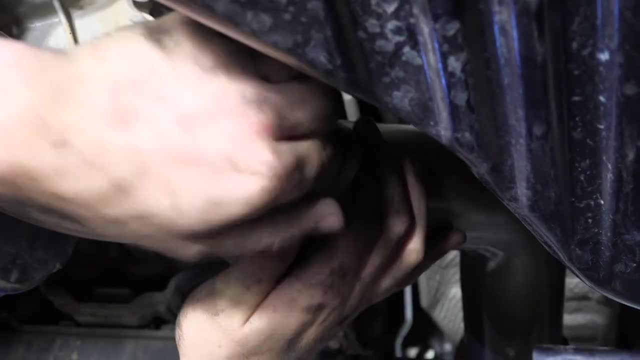 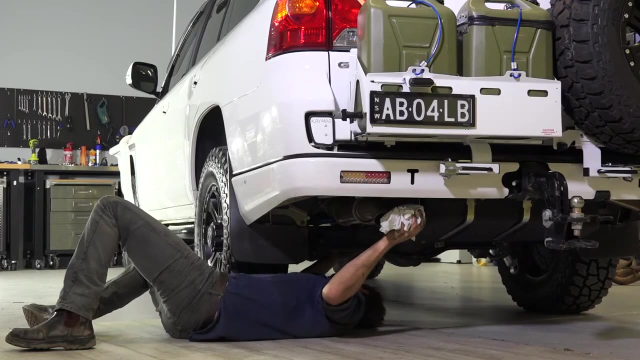 the exhaust into place. Once the exhaust is in, go back and tighten everything up, then you can check for leaks. Put a rag on the end of the exhaust, then get a mate to rev it a bit and listen out for any escaping exhaust. That's how easy it is to install and exhaust. 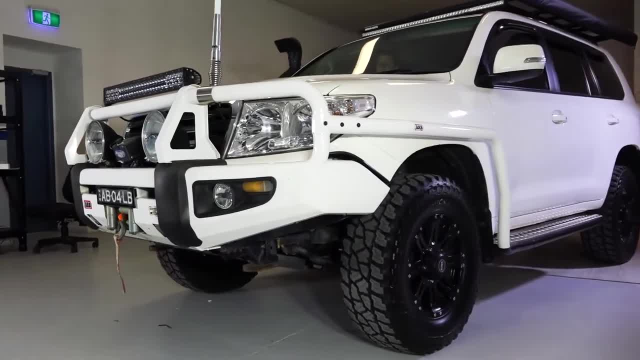 home. now it's time to go for a drive and listen to this big 200 sing. 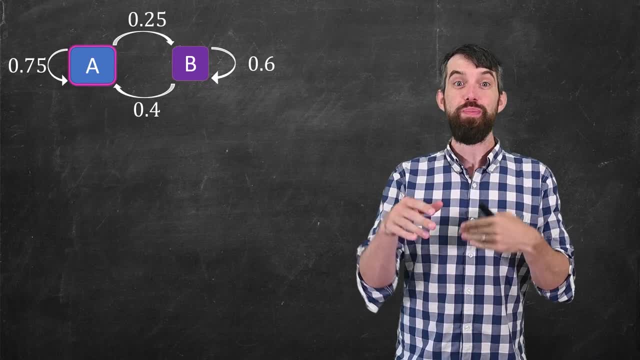 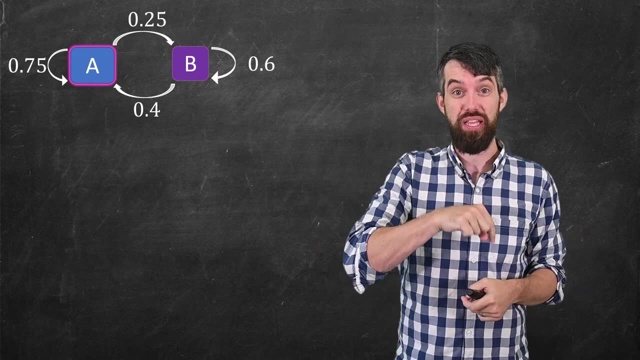 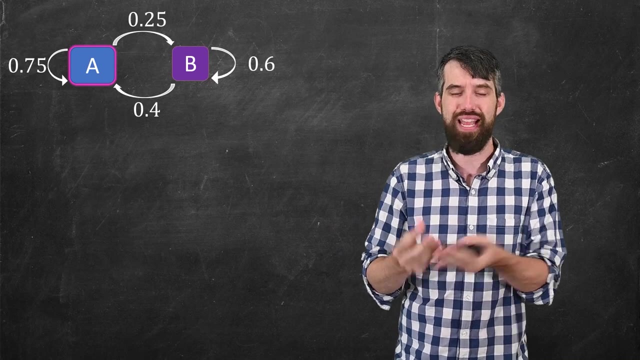 This video is my second video on Markov chains And if you haven't seen the first video on Markov chains, check out the link down in the description. In this video we're going to use some formalisms of linear algebra, the idea of matrices, the idea of vectors and how to multiply those. 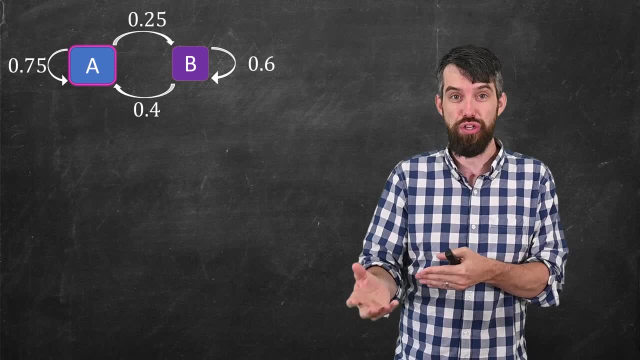 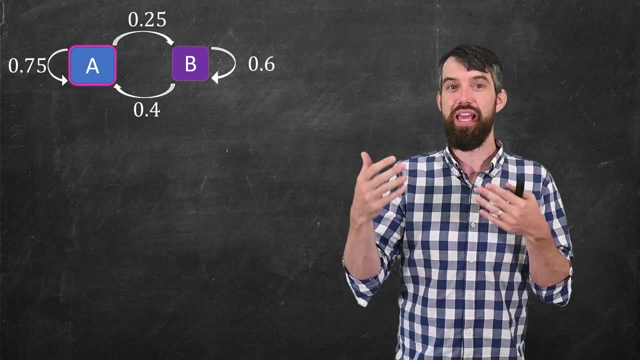 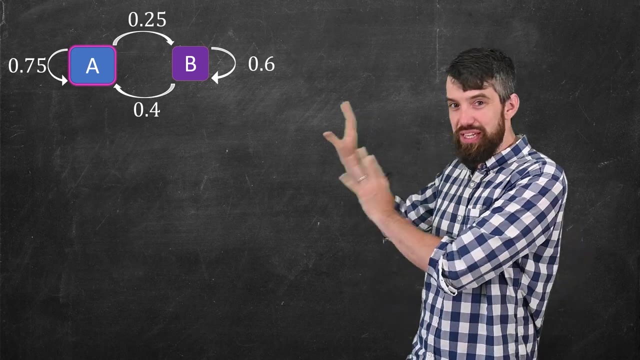 to make the kinds of manipulations that we need to do when studying a Markov chain much, much simpler. Indeed, in the introduction video, we ended with a computational difficulty that we're going to solve in this particular video. So here's the idea. Imagine I have a transition diagram. 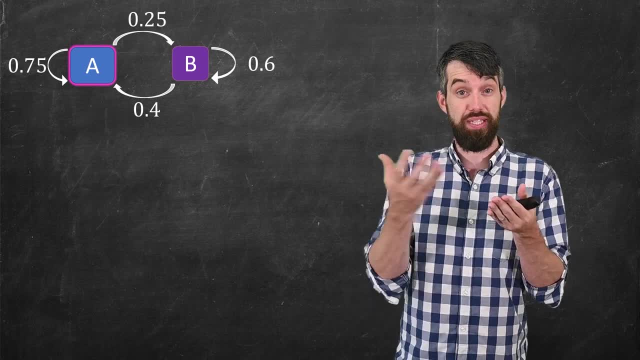 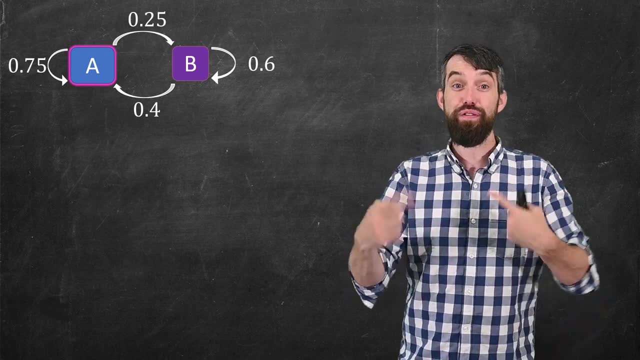 That's what this is. A transition diagram lists the possible states of some systems. So in this example it might be in state A or state B, And then there's a bunch of arrows between those states and the numbers on each arrow describe the probability. So for example, the 0.75 that 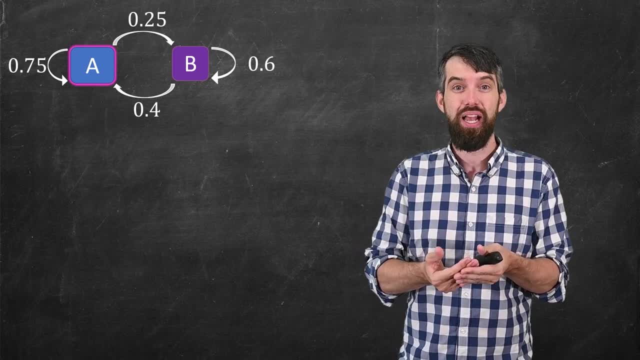 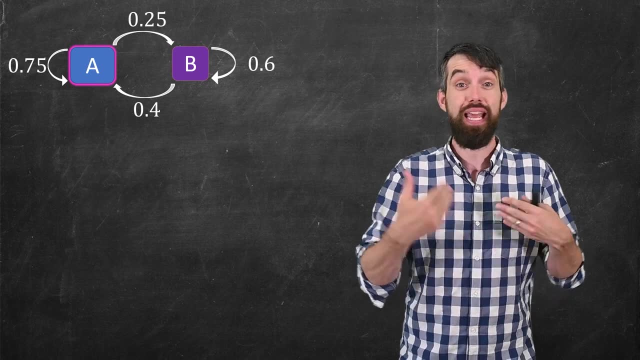 is on the arrow is 0.75.. And then there's a bunch of arrows between those states, and the numbers on each arrow that goes from state A to state A represents that there's a 75% probability that state A in one iteration is going to transition to being state A in the next. So what I'm going to do 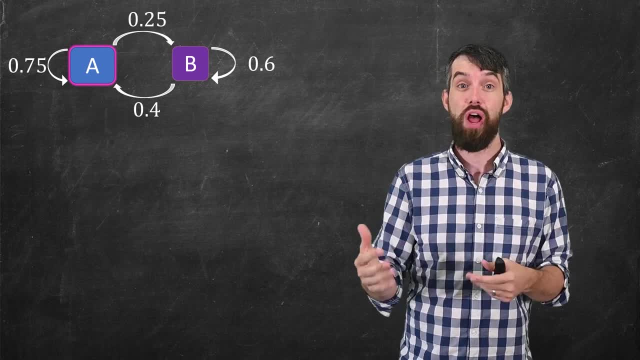 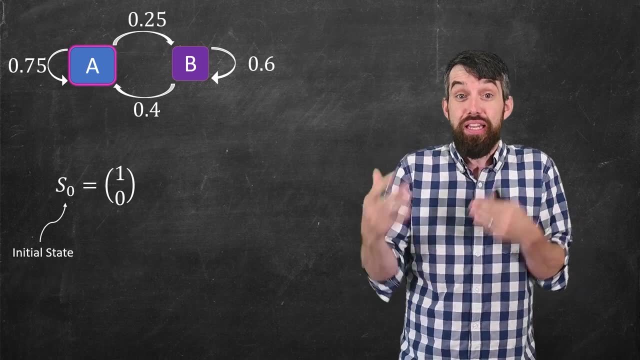 first is introduce some notation to help me describe different things. The first is going to be what I will call S0. And this is referred to as the initial state of the system And it's a vector. It's got a 1 and a 0. So what does that mean? So, basically, 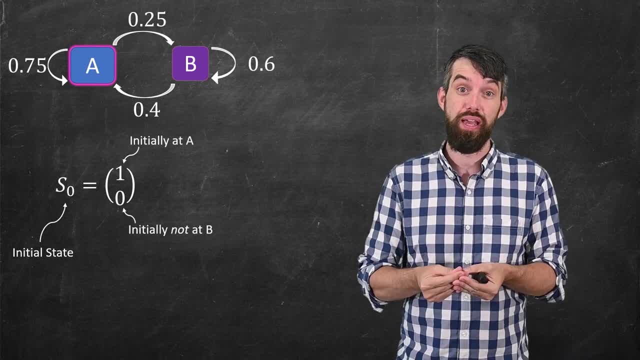 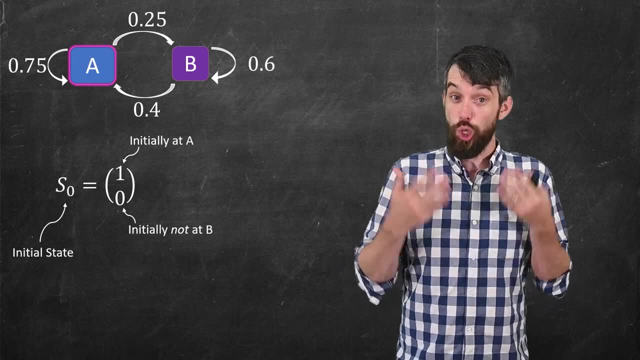 the top component of my vector refers to state A and the bottom component to state B. If you had more components in your system- A, B, C, for example- then you'd have three components in your vector And the fact that it says 1 and 0 means there's a 100% probability that it starts.